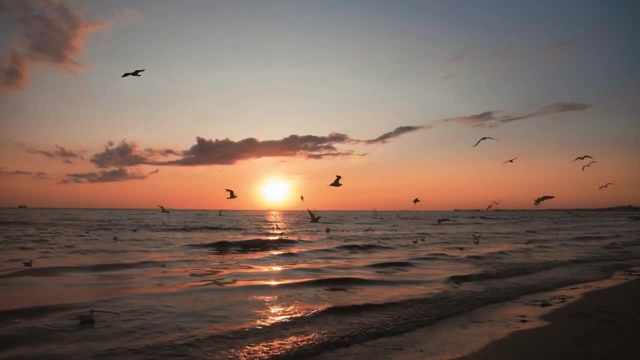 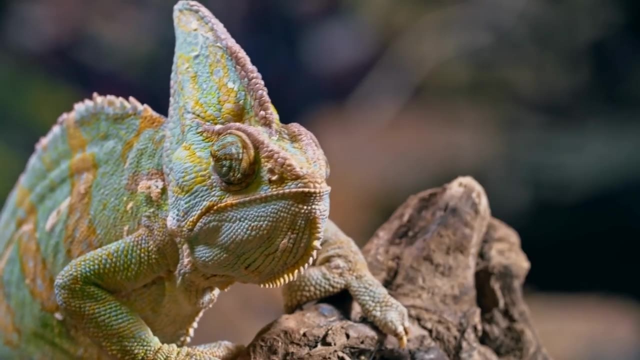 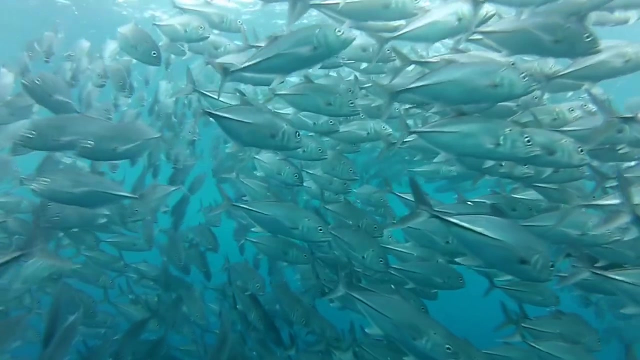 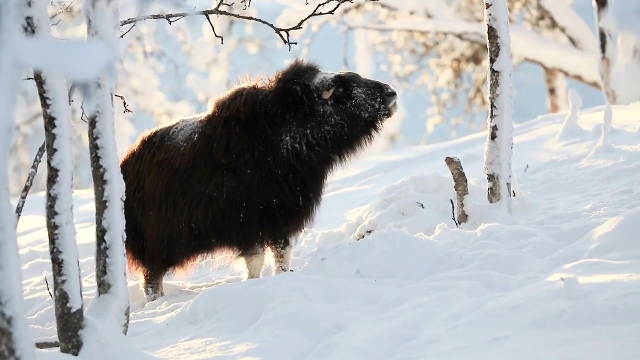 and lifeforms. The biosphere is all about life. It encompasses all regions of the Earth where life exists, from the deepest parts of the ocean to the highest mountains, from the chilliest arctic regions to the hottest deserts and everything in between. 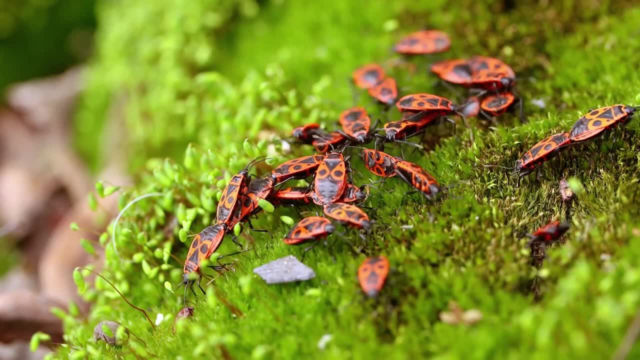 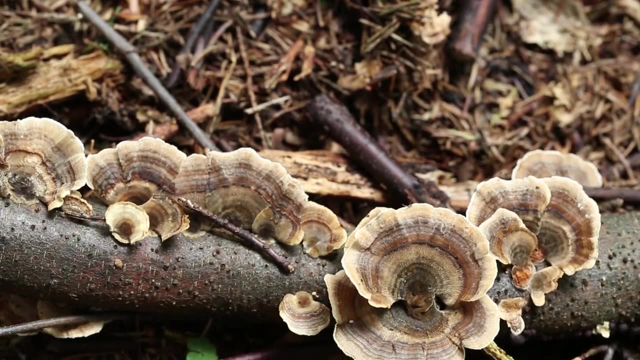 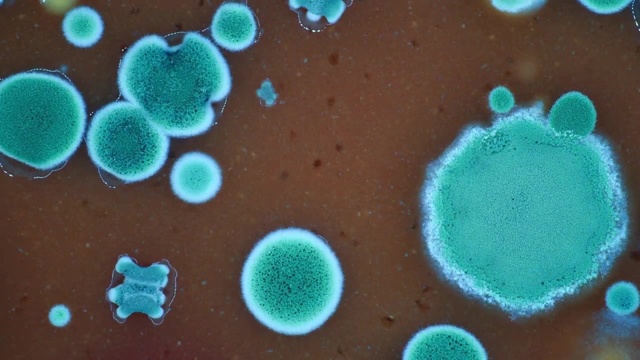 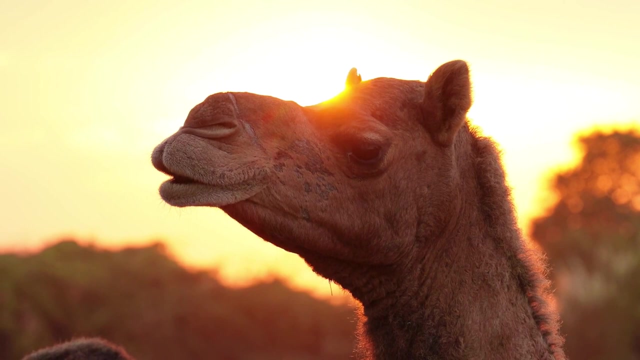 The biosphere encompasses all forms of life on Earth. This includes not just animals and plants, but also fungi, bacteria and various other microorganisms that might not be visible to the naked eye. In the desert regions, we have organisms such as cacti and camels, which have adapted to 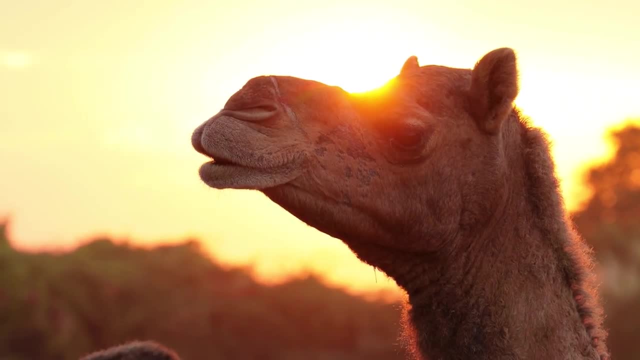 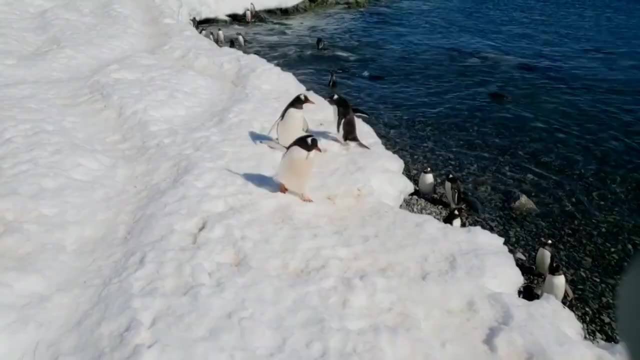 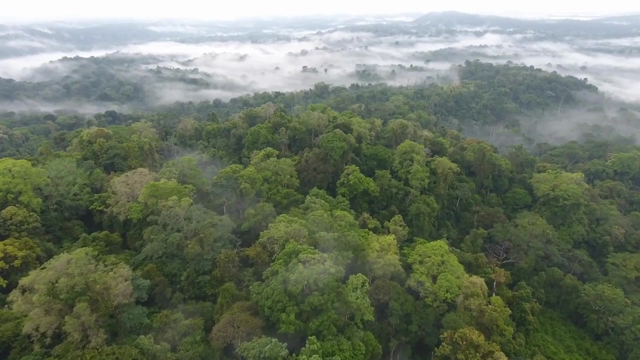 the extremely dry and hot conditions In the polar regions… In the polar regions… In the polar regions… Polar bears… Polar bears… Penguins… Penguins… Various species of seals thrive in the cold environmental project Forests, which can range from tropical rainforests near the equator to boreal forests closer. 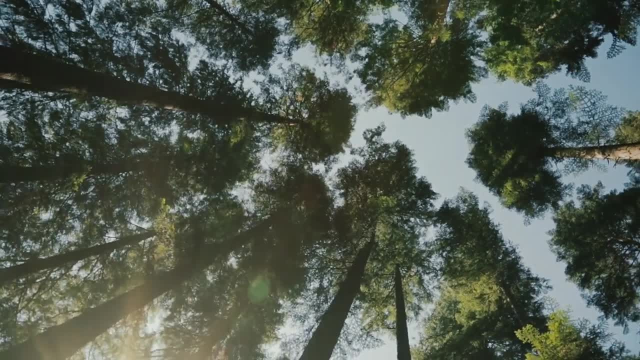 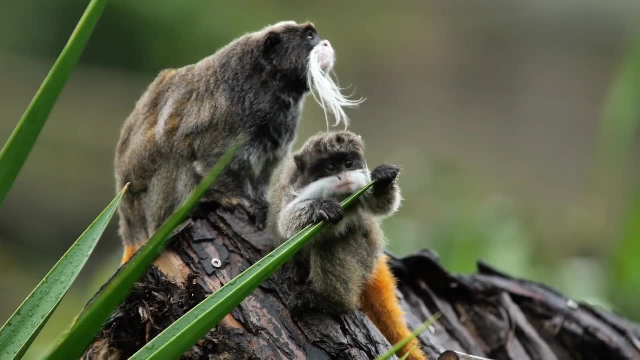 to the poles, host a diverse array of life, From towering trees- Desde tien fe, Styrie抑en groans and understory plants to a myriad animals such as monkey, green lemons, birds, birds, satellites- still most immigrants, Moles, aborigines, kişiklings, karr estamos. birds, deer, wolves and countless insects. The biosphere also spans aquatic regions, both fresh and saltwater. Coral reefs, for instance, are teeming with life, from the corals themselves to the numerous species of fish, crustaceans and other sea life they host. 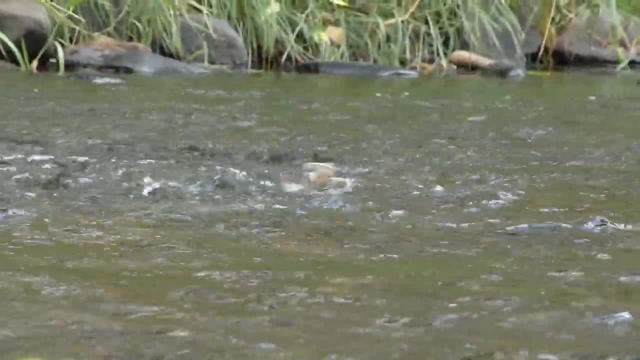 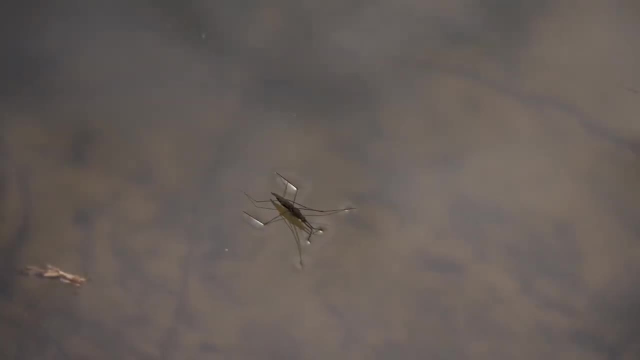 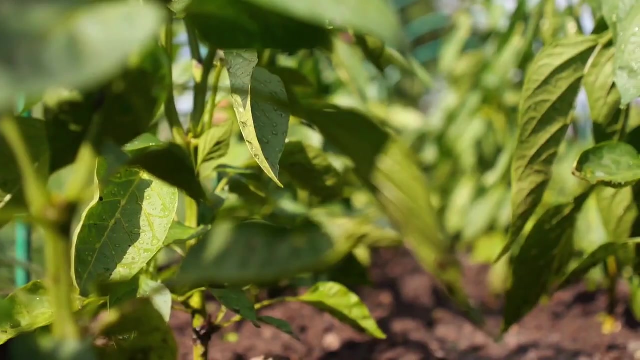 Freshwater ecosystems like lakes and rivers are home to fish, amphibians, waterfowl and many other types of invertebrates. The biosphere interacts with the other spheres in numerous ways. Plants grow in soil, which is a part of the geosphere. 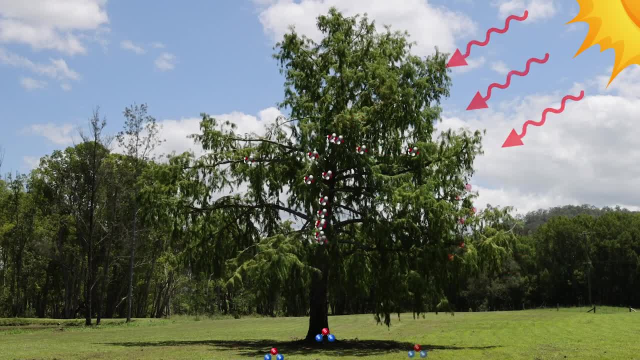 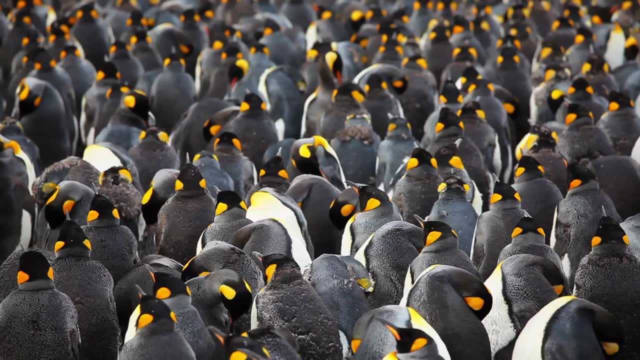 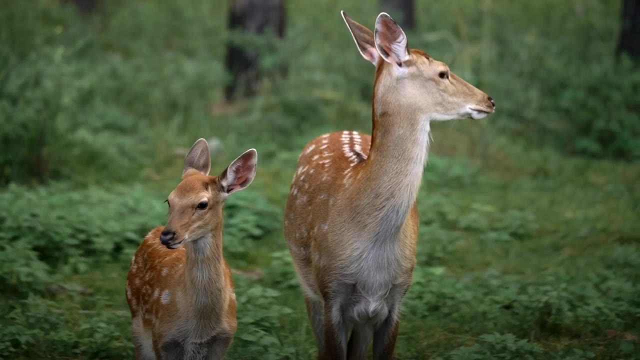 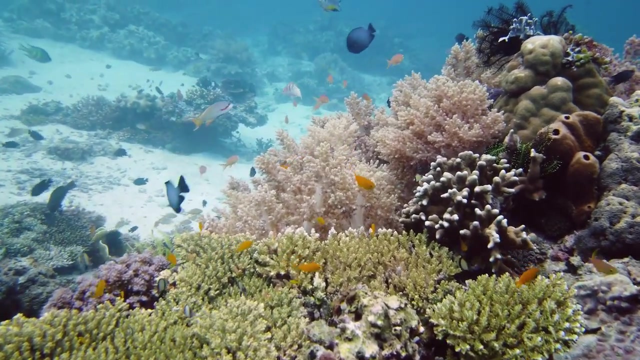 They take up carbon dioxide, which is a part of the atmosphere, and require water, which is a part of the hydrosphere. Animals breathe in oxygen from the atmosphere and drink water from the hydrosphere. The geosphere and hydrosphere also provide habitats to a great diversity of organisms. 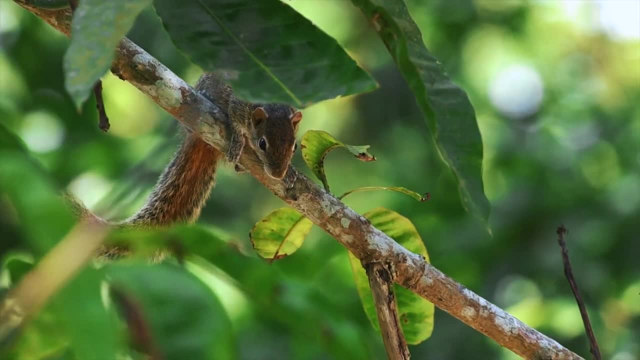 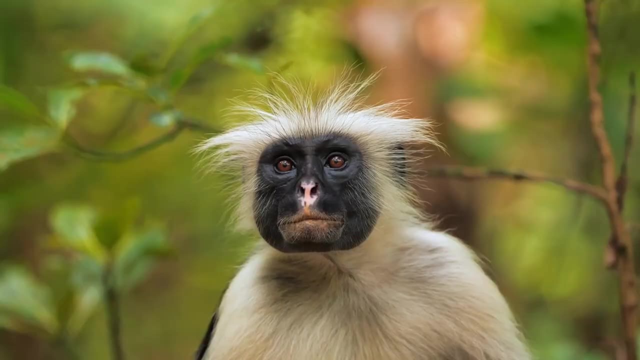 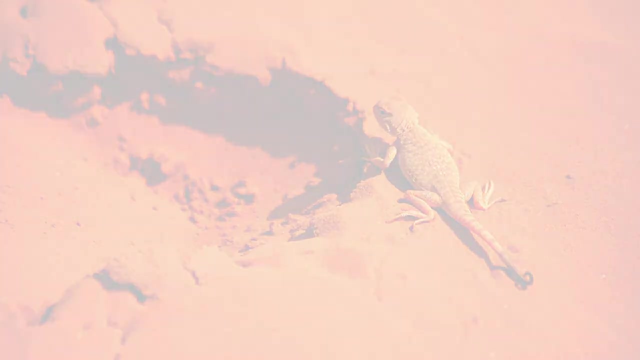 The essential interplay between the biosphere and the other spheres is key. The interdependence of all these spheres illustrates the remarkable balance and interconnectivity of our planet. 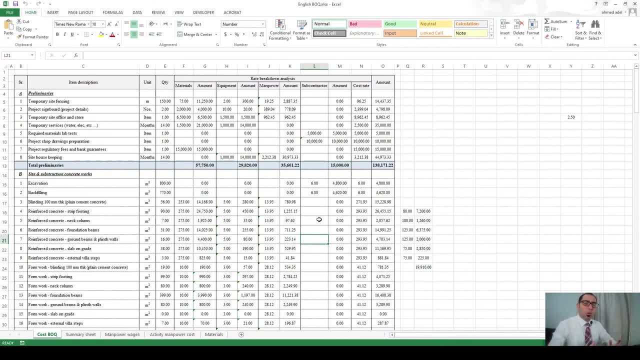 Now I want to explain a little bit about cost estimation. What is cost estimation, guys? Cost estimation, in the simplest way, is that we want to understand how much the project will cost us in general and how much the project will cost us in terms of materials, equipments, manpower. 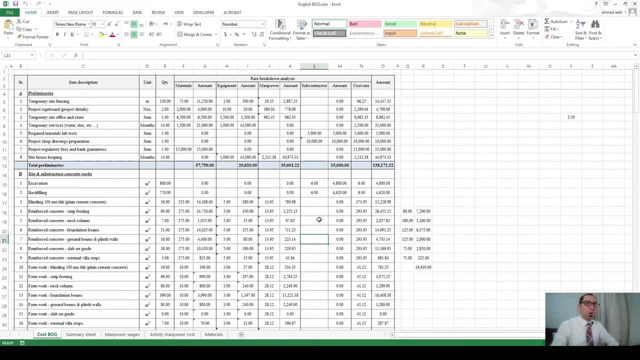 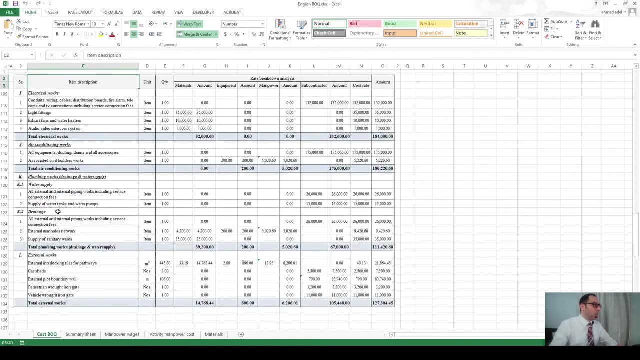 and subcontractor and others. So this is the simplest way to define the cost estimation. So here, if we look at the screen now, if you look at column C, this is the item description and these are the different BOQ items, as you can see. And here is the unit and here is the. 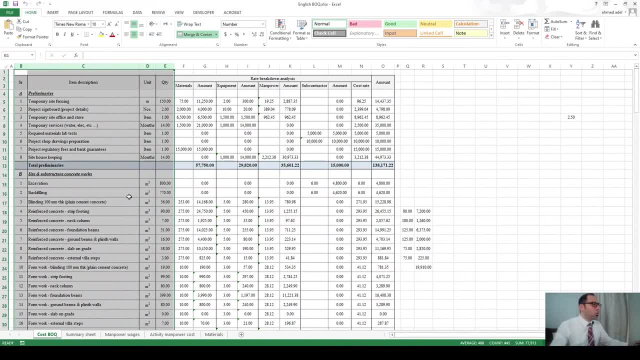 quantity. Up to here. this is a very normal BOQ as we know it. But in the normal BOQ here after the quantity the rate will come, and when the rate multiplied by the quantity you get the amount. But when we are doing a cost estimate, 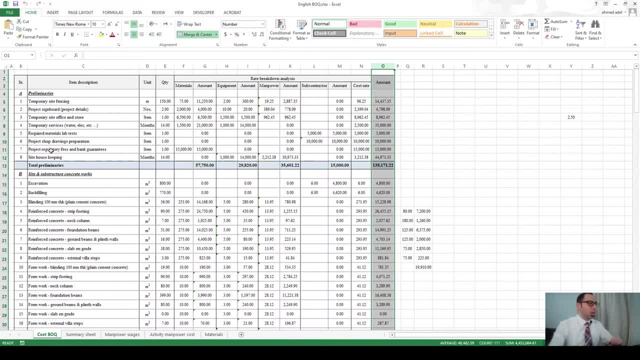 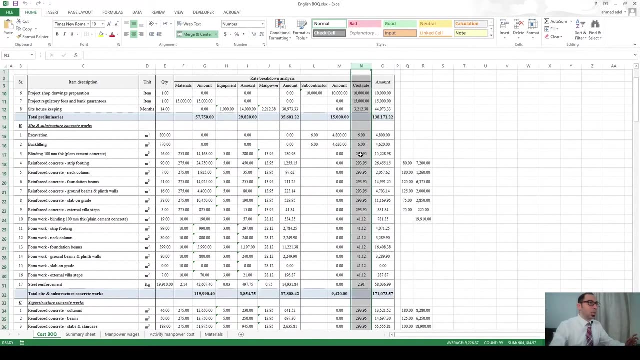 we need to have a little bit more details. And how is that? Now? our rate usually in the BOQ is just one rate, One rate inclusive of materials, equipment, manpower, subcontractor, and we have just one rate. But actually any of these rates, guys- this is the cost rate here- Any of these?